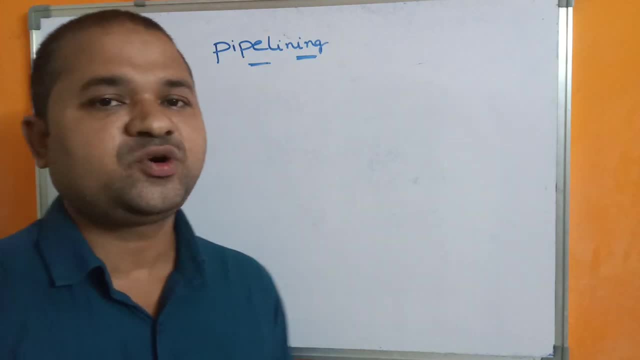 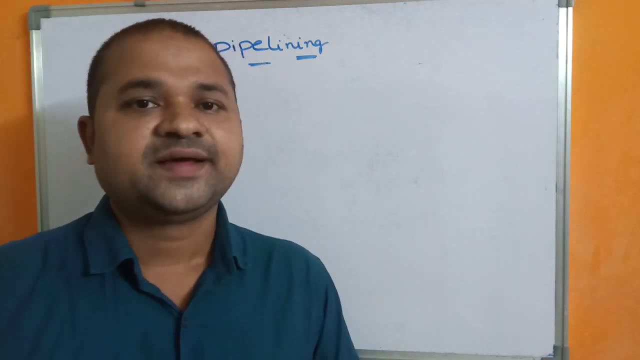 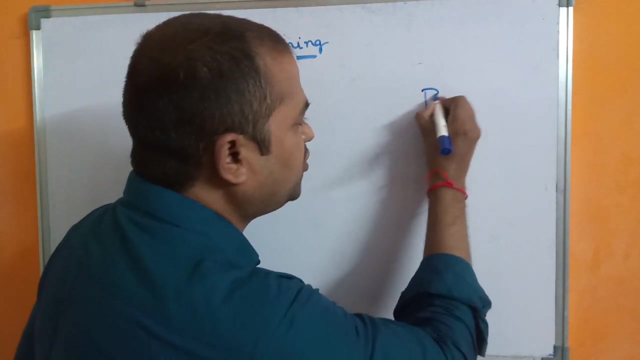 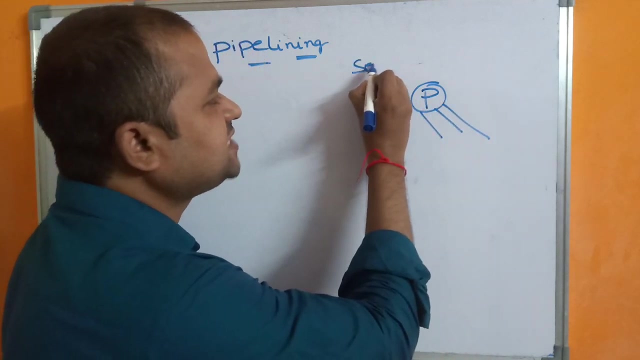 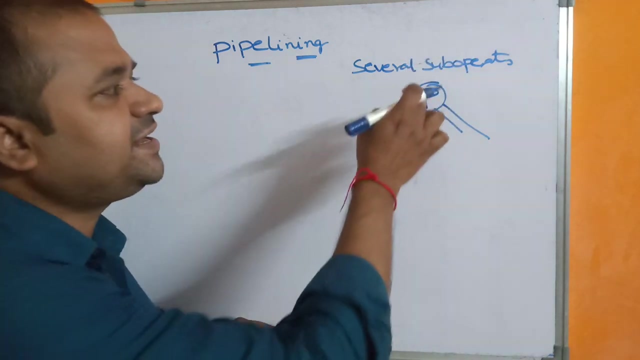 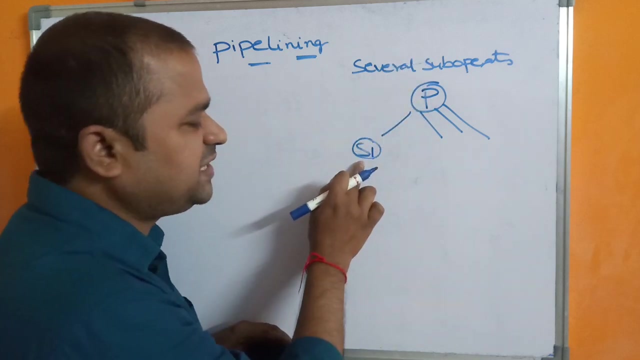 In this video we are going to discuss about pipelining in computer organization architecture. Pipelining means a process is divided into several sub operations, where each sub operation is associated with a segment. The first sub operation represents segment 1, the second sub operation represents segment 2, the third sub operation represents segment 3, and the fourth sub operation represents segment 4.. 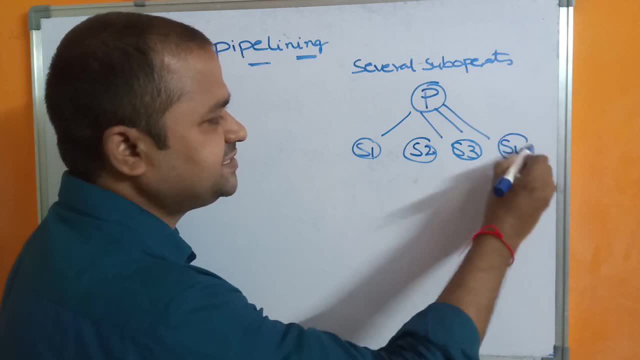 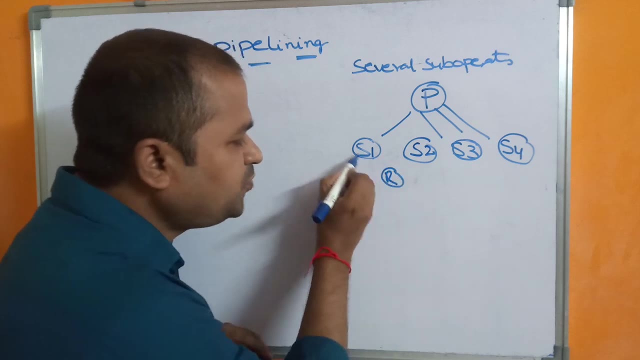 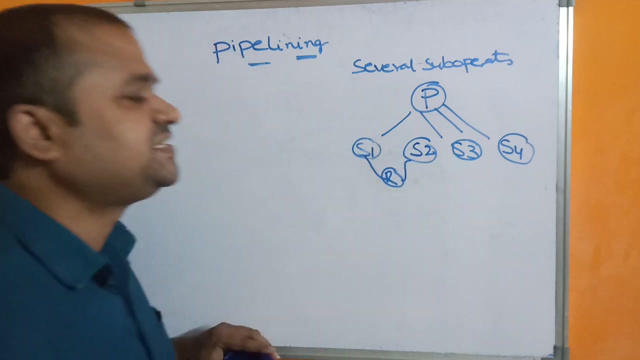 sub-operation represents segment 3, the fourth sub-operation represents segment 4. like that, Here the output of each segment will be stored in a register. So the output of S1 will be stored in a register and this register information is passed as input to the next segment. So 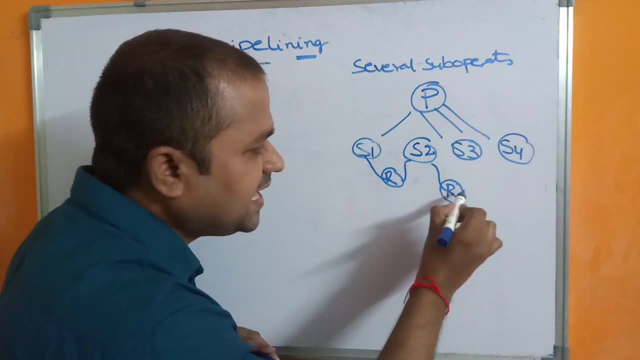 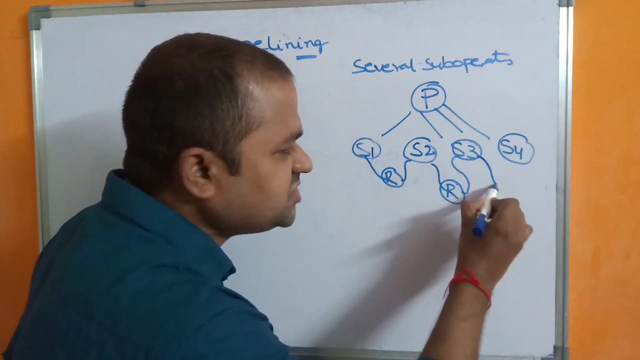 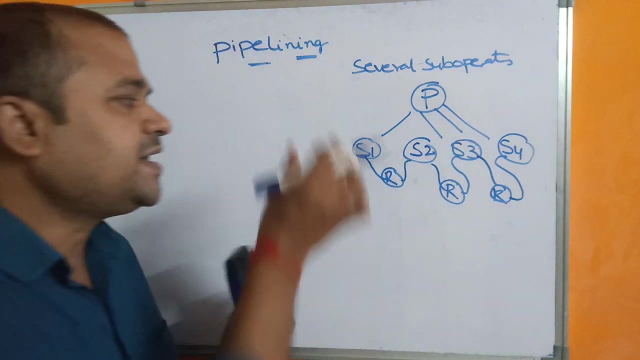 likewise, the output of S2 will be stored in a register and this information is passed as input to the next segment, that is, S3.. And the output of S3 is stored in a register and this information will be passed as input to the segment 4.. Here all the segments will work independently. 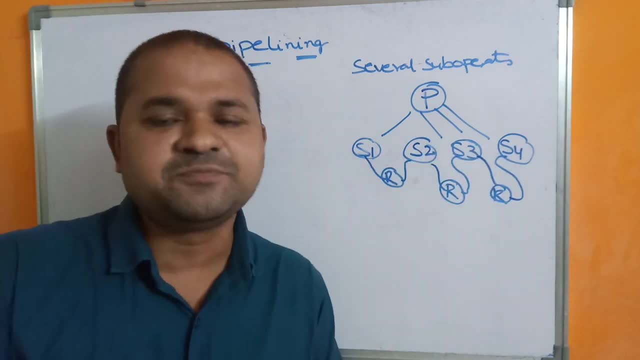 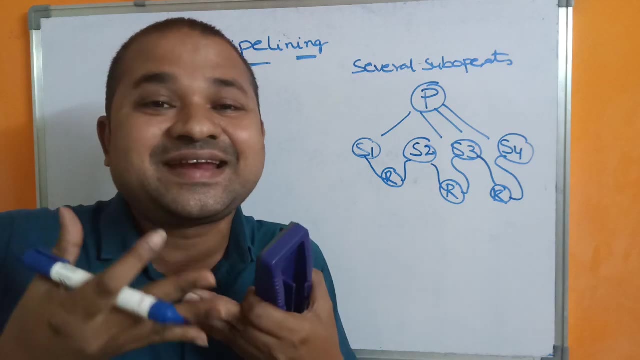 So that means we can execute all the segments concurrently here. So why this is called as pipeline? Why? Because here we are transferring the information from one segment to the next segment. So here we are transferring the information from one segment to the next segment. 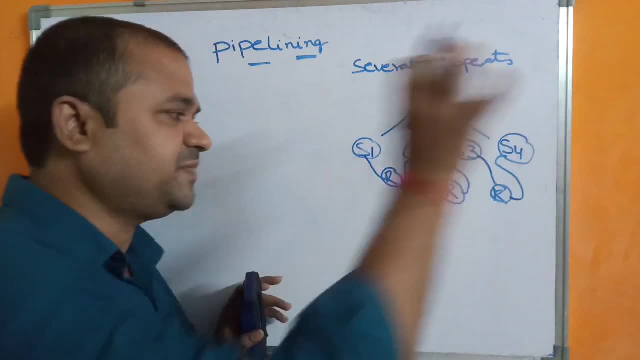 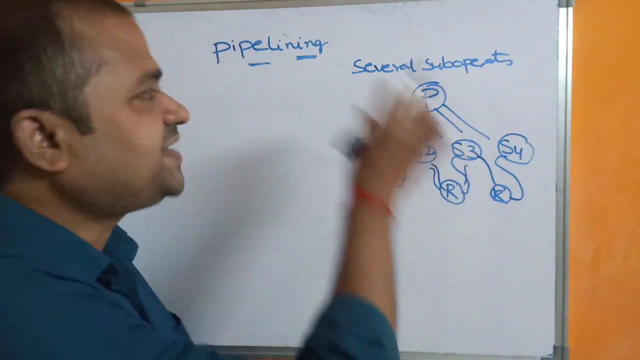 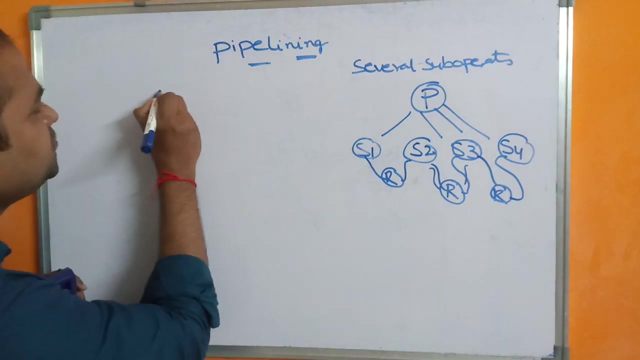 So from S1 to S2, we are transferring some information. From S2 to S3, we are transferring some information just with the help of a pipe like this. So that is why this is called as pipeline. Now let us see an example here. Let us assume 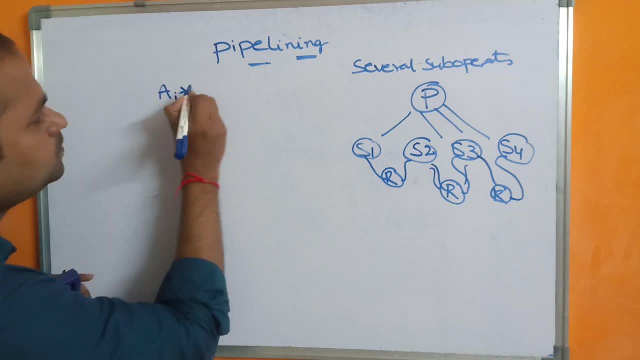 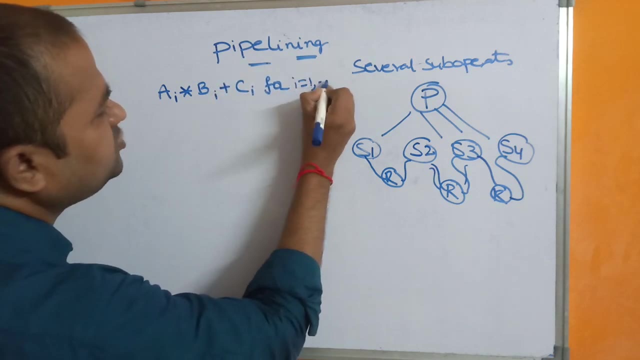 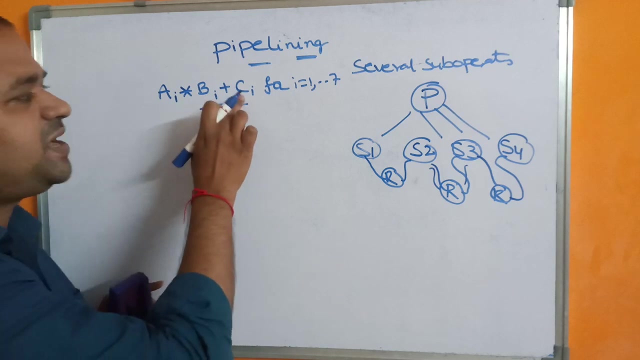 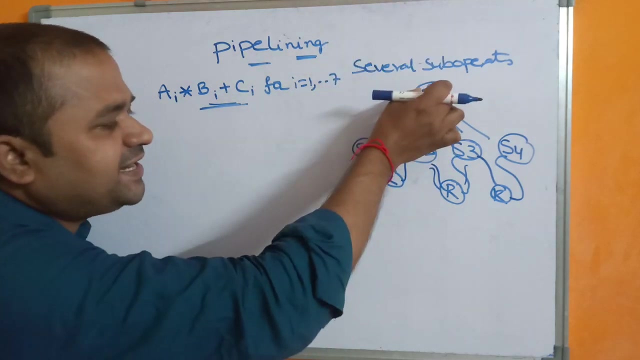 that we have a process: Ai into Bi plus Ci for let the values of Ir from 1 to 7.. So here we have this process. This is our process here: Ai into Bi plus Ci for i is equal to 1 to 7.. So here we know that we have to divide that process into several sub-operations where 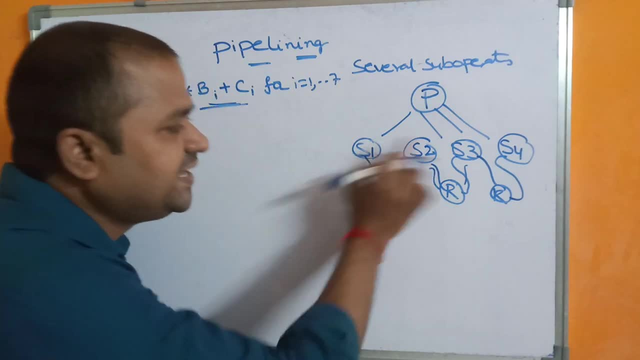 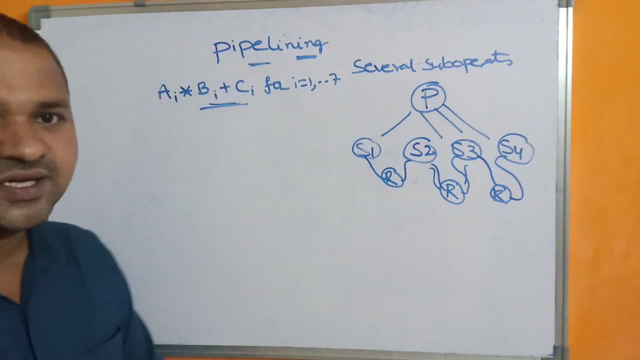 each sub-operation is associated with a segment. So here, the first sub-operation is multiplication, The second sub-operation is addition. So what are the segments that we need here? Here, in order to perform this operation, we require three segments. Segment 1 is nothing. 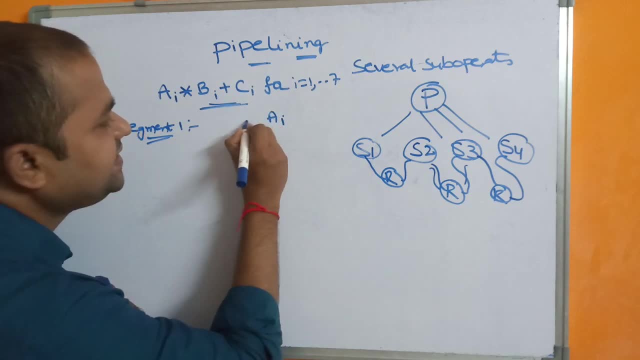 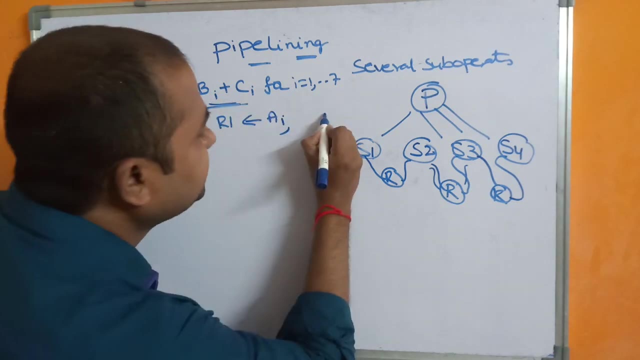 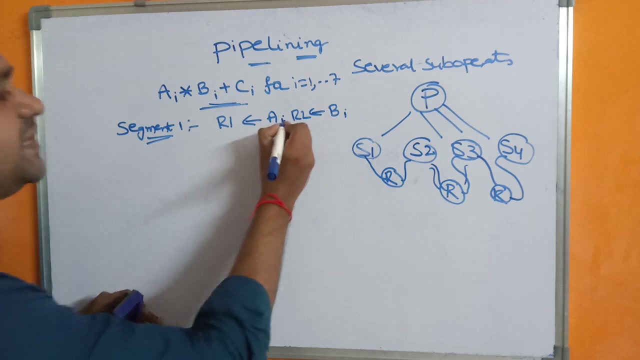 but transfer the content of Ai to a register. Let the first register is R1.. And the second one is we need to transfer the content of Bi to the second register. Let it be R2.. So this is nothing but segment 1.. So in segment 1, Ai content is transferred to other register. 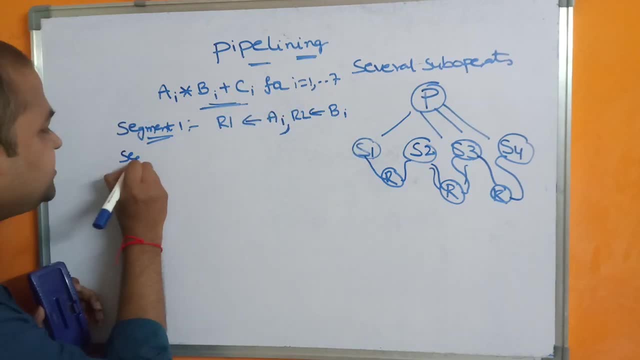 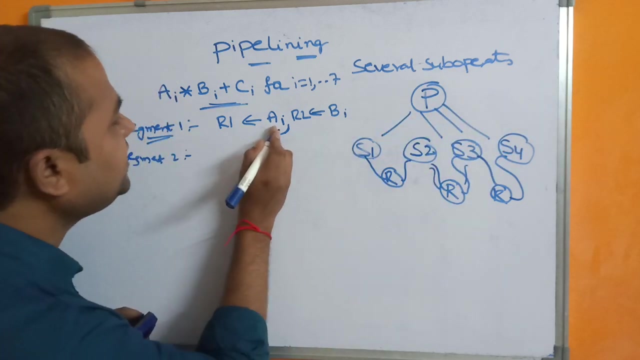 As well as Bi, content is transferred to R2 register. Now let us see about segment 2.. In segment 2, what will happen is multiplication operation will be performed on this. Ai and Bi, as well as Ci, will be loaded into a new register. So here, Ani result is available. 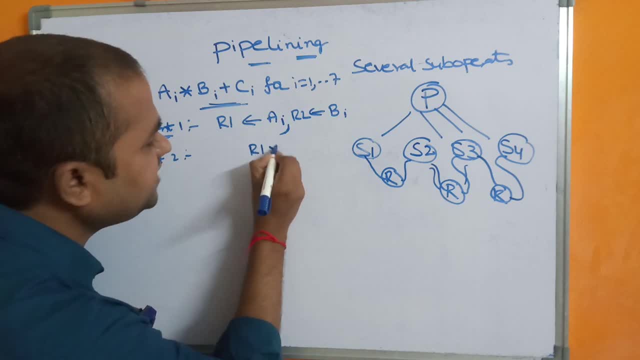 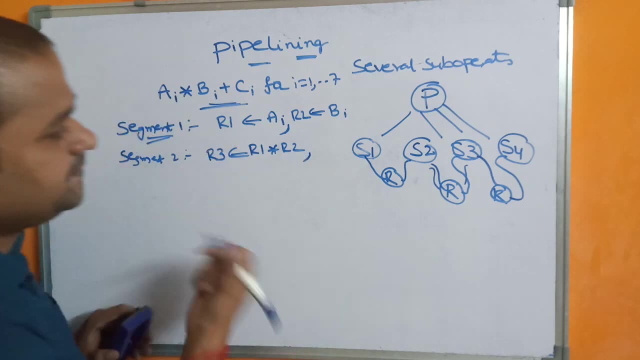 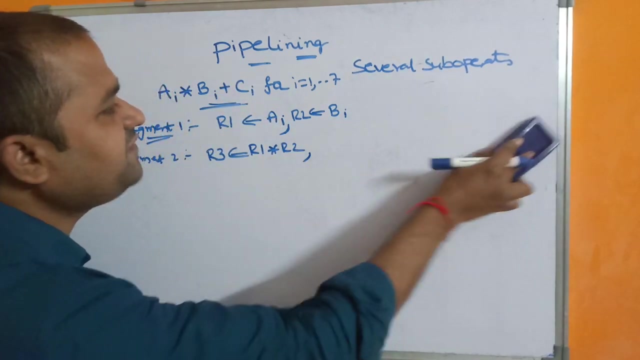 in R1.. Bi result is available in R2.. So multiplication will be performed on R1 and R2.. So we will get Ai into Bi now and the result is transferred to a register called R3.. As well as so, during segment 2, what will happen is that C- i will be loaded into a resistor. 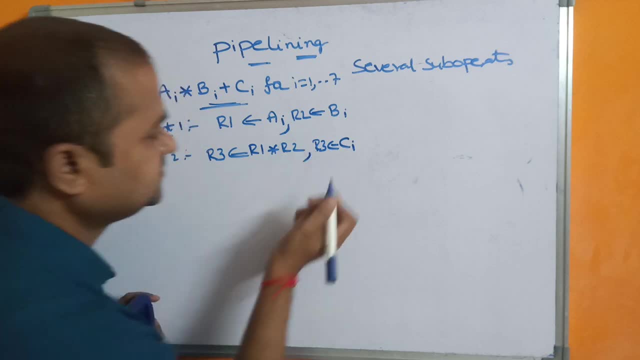 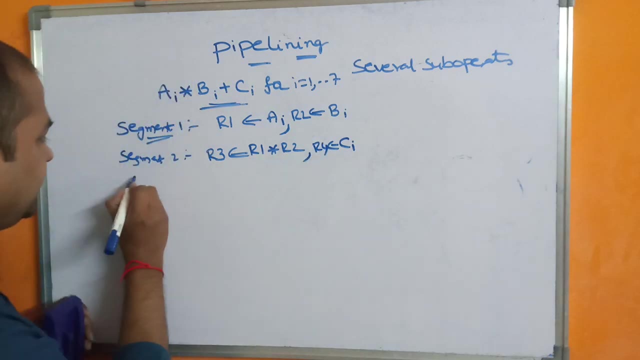 So C i will be loaded into a resistor called R 3, R 3, okay, Already, we have taken R 3.. So what is the next resistor? The next resistor is R 4,- okay, And now let us see about segment 3.. 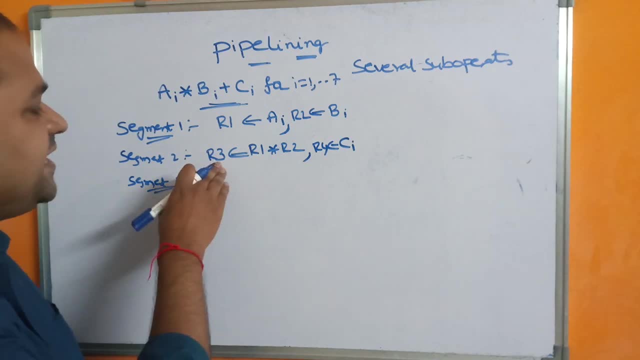 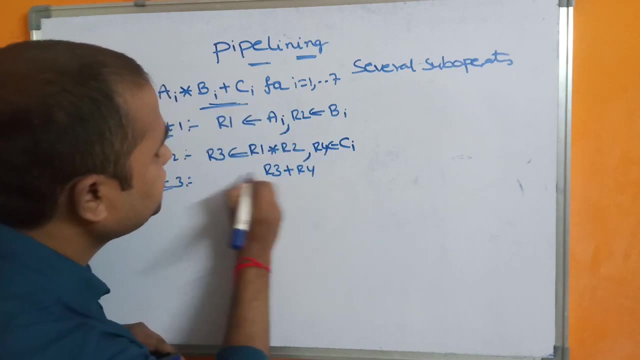 In segment 3, what will happen is already: multiplication result is present in R 3 as well as C i result is present in R 4.. So we have R 3 and R 4.. So transfer the result to R 5.. 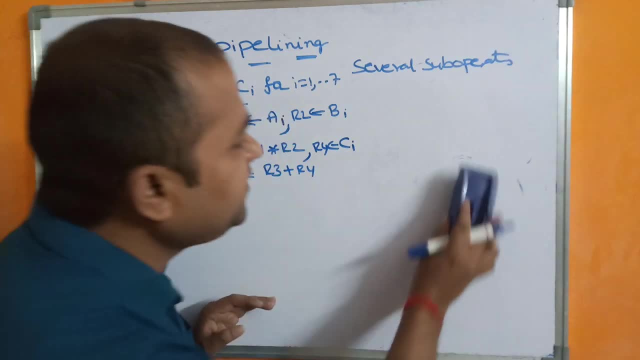 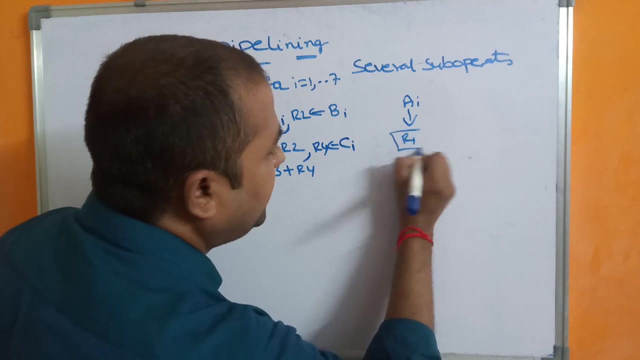 So these three are the segments that we have here. If you want, we can represent this one with the help of a diagram like this. So A i is transferred to R 1, R 1 resistor, as well as B i is transferred to R 2 resistor. 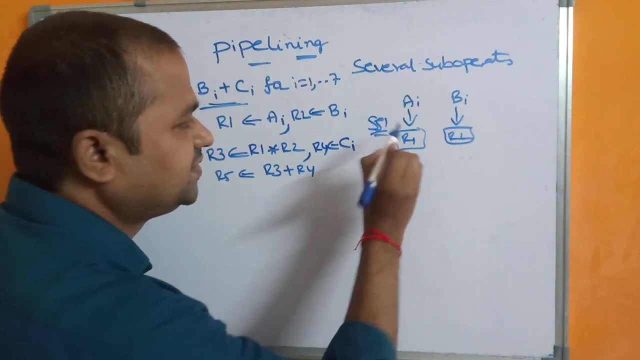 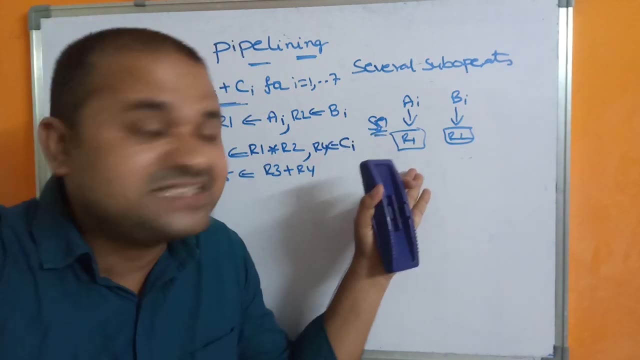 okay, So this is nothing but what Segment 1.. So here what will happen? The output of each segment will be stored. So this is the output of each segment. So the output of each segment will be stored in a resistor and that resistor information. 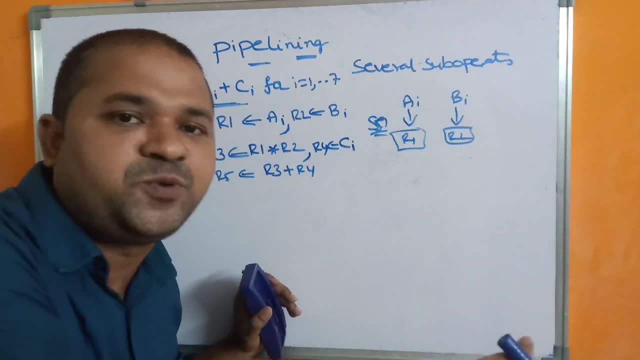 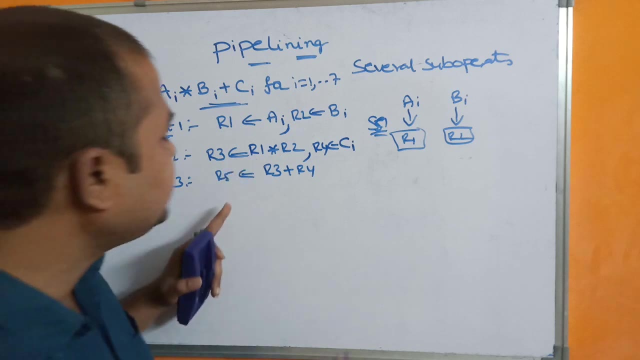 and that information will be passed as input to the next segment. So what is the next segment here? R 1 and R 2 will be multiplied and the result is transferred to R 3. So here we have to take a combinational circuit. 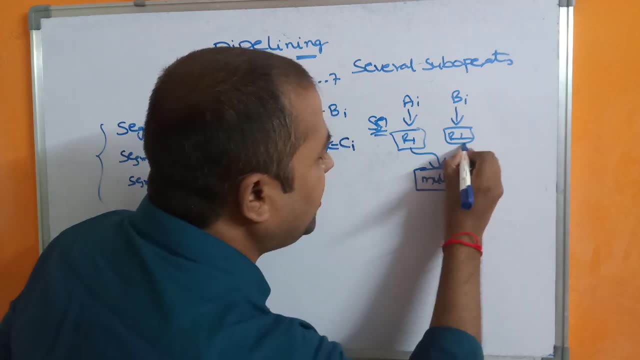 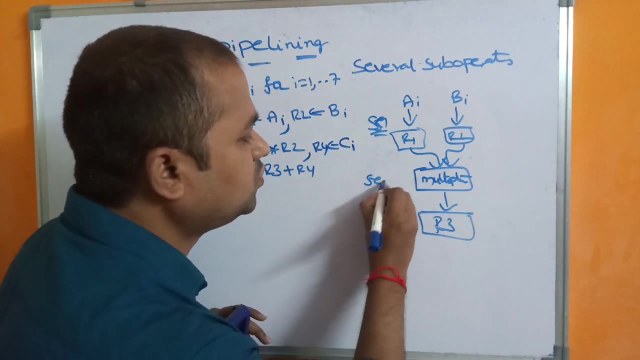 So this is nothing but multiplier. So multiplier multiplies R 1 and R 2 and the result is transferred to which resistor R 3. So this is what Segment 2.. So in segment 2 also. 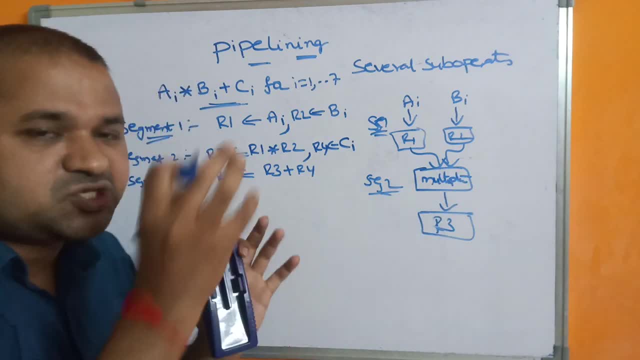 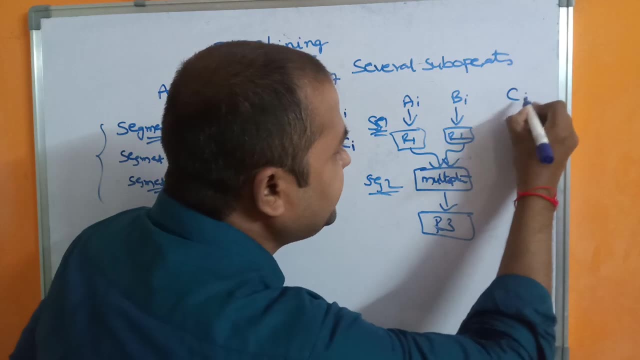 The output of this multiplication is stored in a resistor. okay, So the output of each and every segment is to be stored in a resistor, as well as what will happen here. C i content is transferred to R 4 resistor. okay, So next to what will happen. 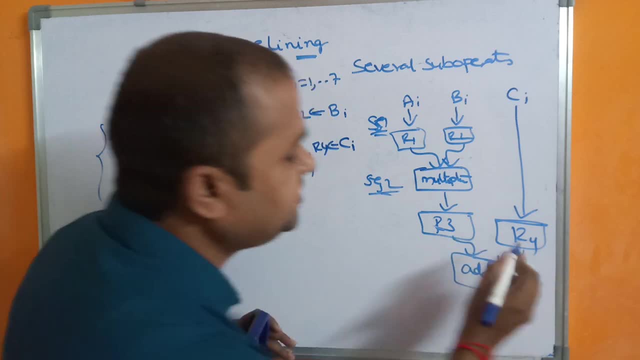 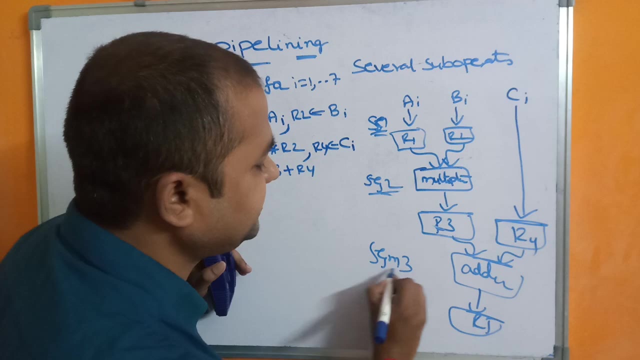 Yarder performs addition operation on R 3 and R 4 and the result is transferred to R 5 resistor. okay, So this is nothing but segment 3.. Segment 3.. So the output of the yarder is stored in a resistor called R. 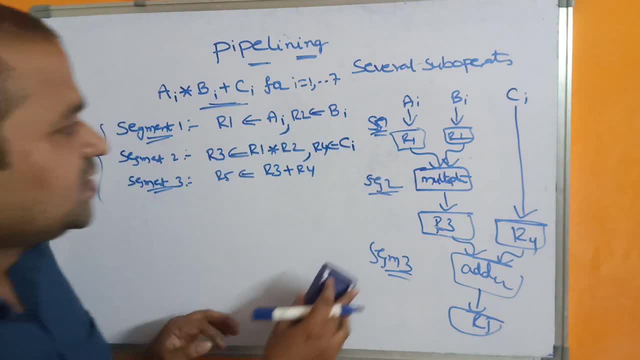 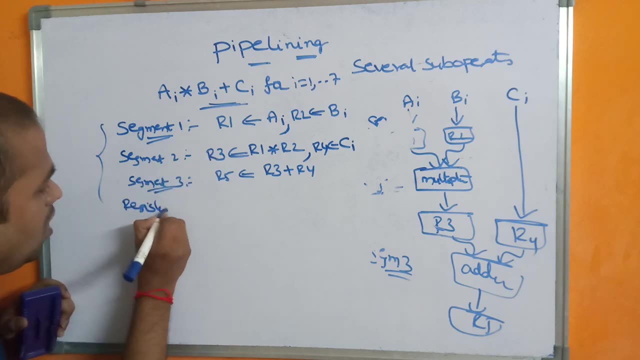 So with the help of this diagram, we can represent like this: Now let us see the resistors here. Let us see the resistors here, So how we can execute this long process with the help of some resistors. Let us assume that here we have how many segments. 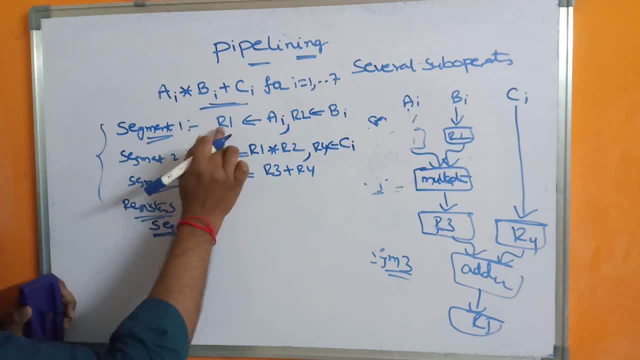 We have three segments. So segment 1 contains how many resistors? In segment 1, we need to maintain two resistors: R 1 and R 2.. In segment 2, what are the resistors We need to maintain? R 3 and R 4.. 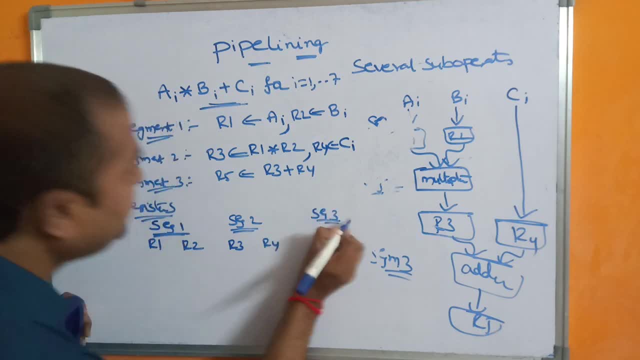 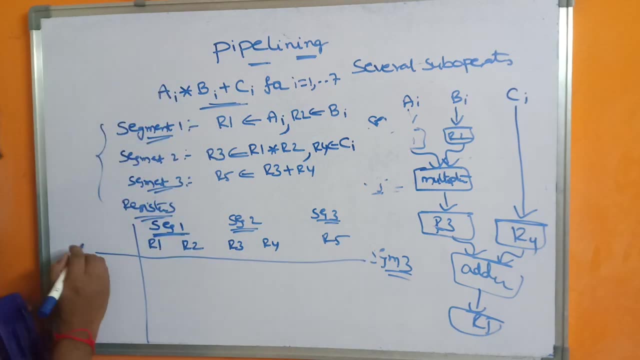 R 3 and R 4.. And in segment 3,, what are the resistors? We have only one resistor, that is R 5.. So now let us see how this will be executed. So here it represents clock cycle. here. 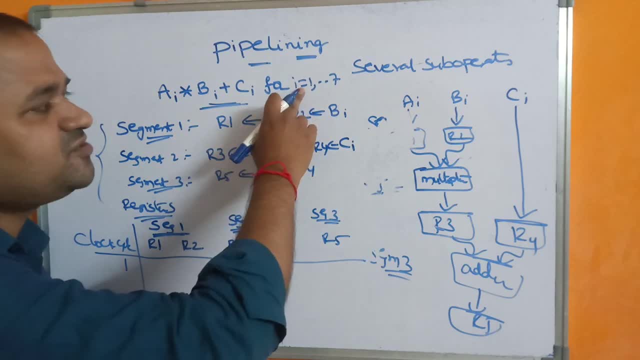 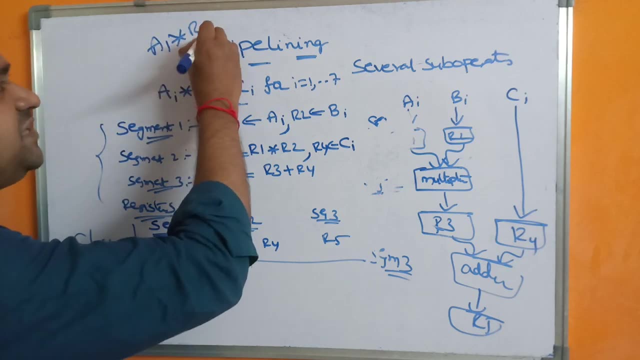 In the first clock cycle. what will happen is here: what are the I values? I values are from 1 to 7.. So we have to execute instructions like A 1 into B 1 plus C 1.. So this is our. 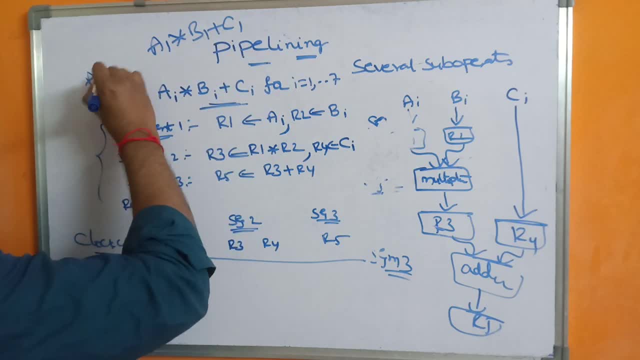 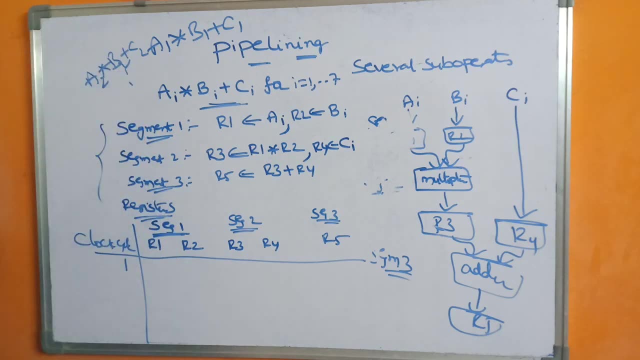 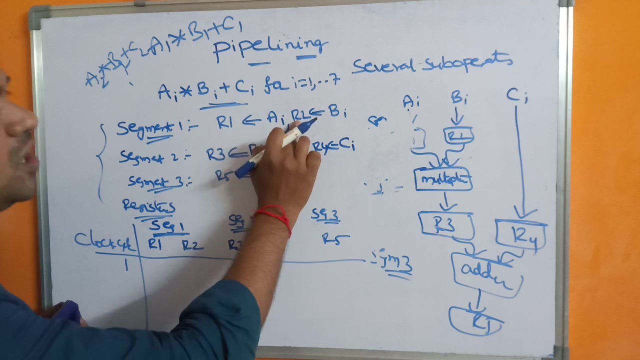 our first output And the second output is A2 into B2 plus C2.. So likewise we need to produce the outputs up to A7 into B7 plus C7.. So in the first class cycle what will happen is A1 is loaded to R1 as well as B1 is loaded to R2.. Why? Because the initial 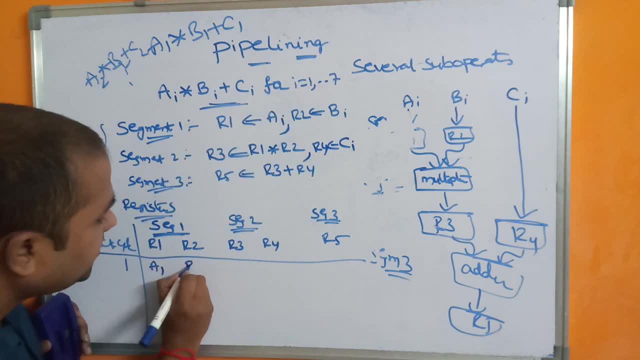 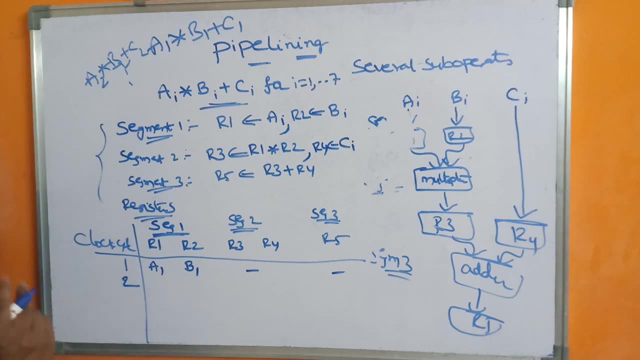 value of I is 1 here, So A1 is loaded to R1, B1 is loaded to R2.. So nothing will happen in segment 2 and segment 3.. Now let us see the second clock cycle. In the second clock, 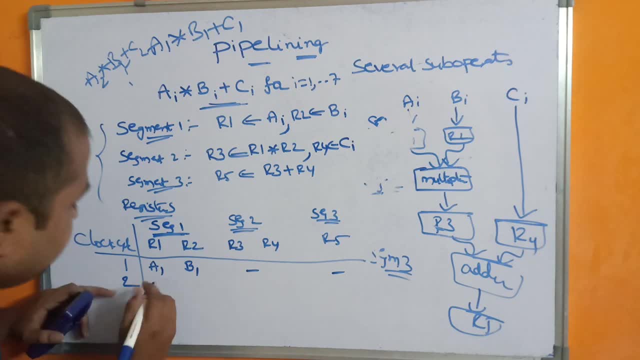 cycle. what will happen? Let us see the second clock cycle. In the second clock cycle, so in the first segment, what will happen is so: what is the next time? value 2.. So A2 will be loaded to R1 as well as B2 will be loaded to R2.. Next, let us see the second. 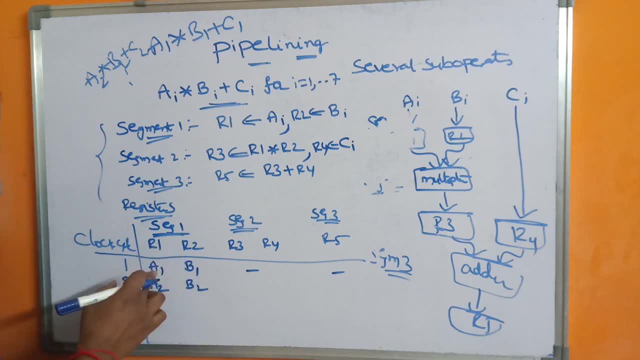 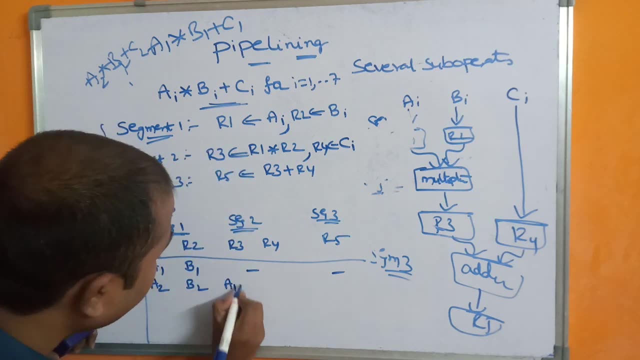 segment 2. here Already in segment 1 we have A1 is present in R1 as well as B1 is present in R2.. So we can multiply those two here, So A1 into B1, A1 into B1.. So R3 means what A1 into? 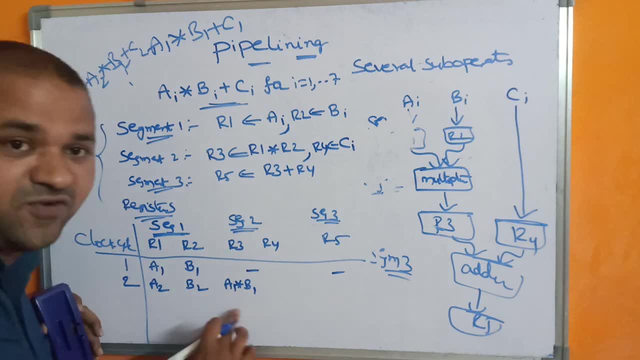 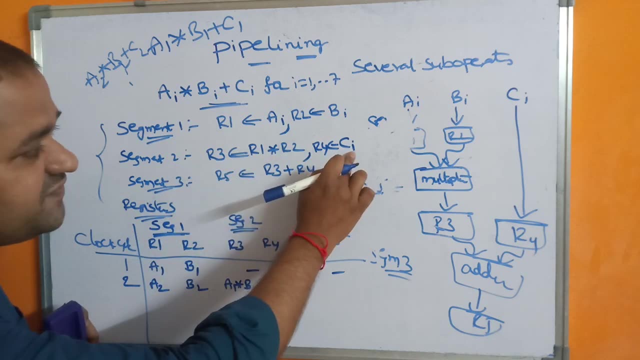 B1. So that here we are representing the information in the form of A and A, B and C, here as well as Z. So what is? second segment? So C1 will be loaded to C1 will be loaded to R4. So C1 will be loaded to R2, R4. So nothing will happen in segment 3.. In the third, 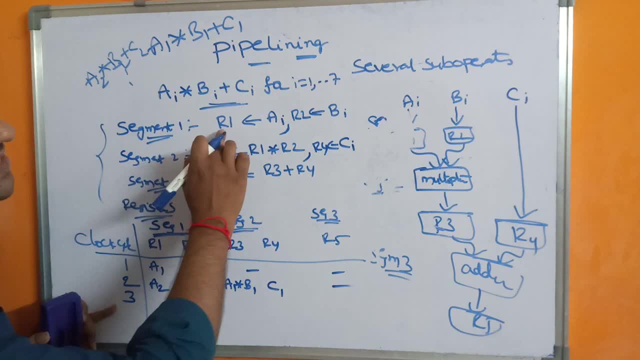 clock cycle. let us see the third clock cycle. So first. first let us see about segment 1.. So A3 will be loaded to R1, B3 will be loaded to R2.. Next, coming to the second segment, so what will happen is A2 and B2 will be. 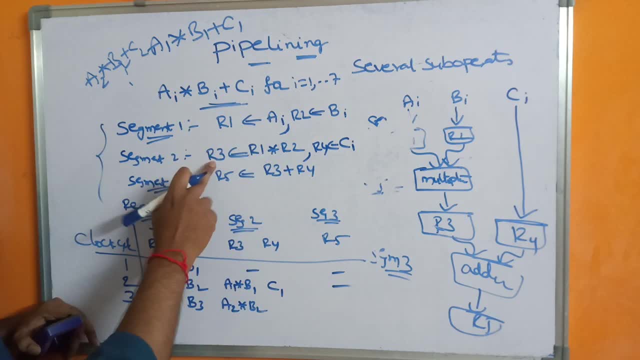 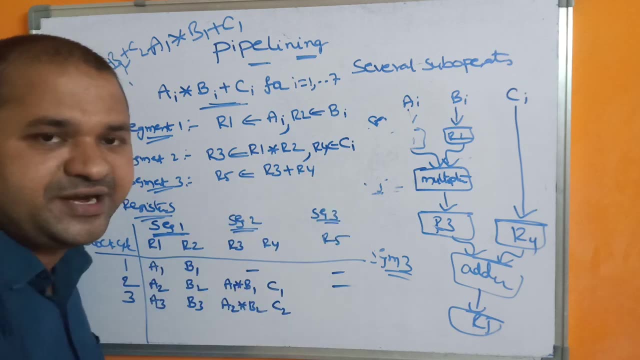 multiplied. A2 and B2 will be multiplied and the result is stored in R3 register as well as the C2 is loaded into R4 register. C2 is loaded into R4 register. Now let us see the third segment. So what is the third segment? We have to add the C2 into R4 register, So 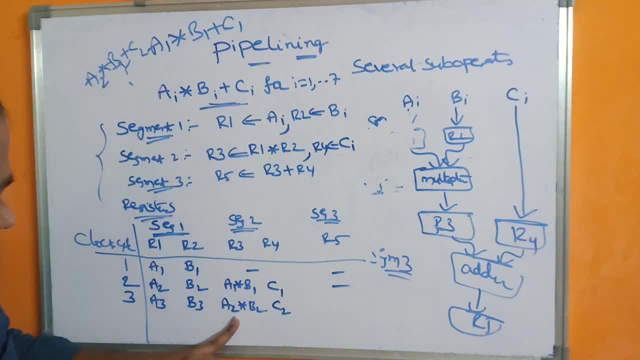 we have to add R3 and R4. So R3 means what? So R3 means this one: A1 into B1, A1 into B1 plus C1. So during the third clock cycle we got the first output. So now we can say: 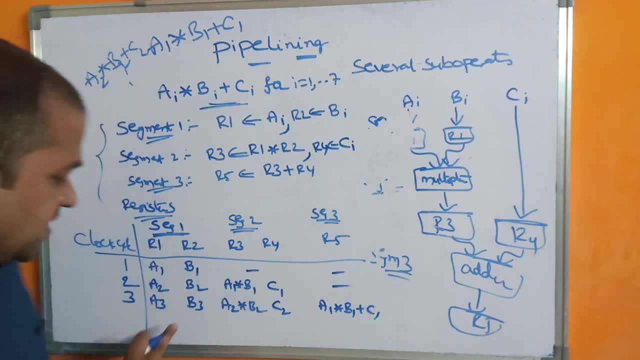 that the entire pipeline is completely filled. Segment 1 contains some data. segment 2 contains some data. segment 3 contains some data. Now, during fourth clock cycle, what will happen? A4 is loaded to segment 1, C2 is loaded to C3.. Now what will happen? A4 is loaded to segment 1, C2 is loaded to C3.. Now what will happen? A4 is loaded to segment 1, C2 is loaded to C3.. Now what will happen? C3 is loaded to section 1, C4 is loaded to section 2, and. A4 is loaded to section 3.. Now, when second loop runs through segment 1, C3 will be loaded to R1,. B1 is loaded to R4.. Now, how long will it take the loop? wait a minute. The 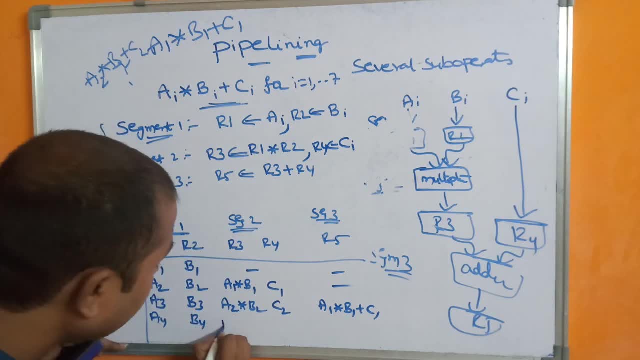 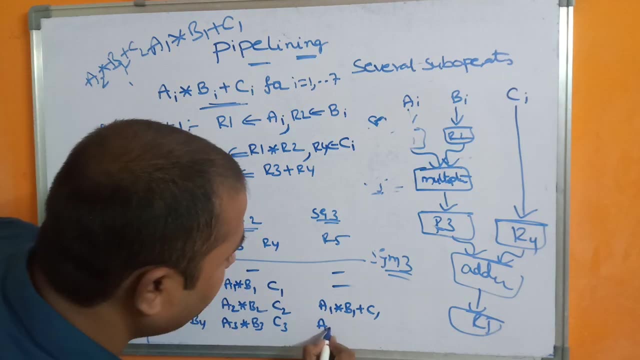 next loop will be like this…. Go ahead and do it same way. A4 is loaded to R1, B1 is loaded to C3.. B1 is loaded to A4.. Now we got the Cgo and Dgo back. So now we got the Cgo, B2 is loaded to C3. And hit the Dgo. So now, if we add, 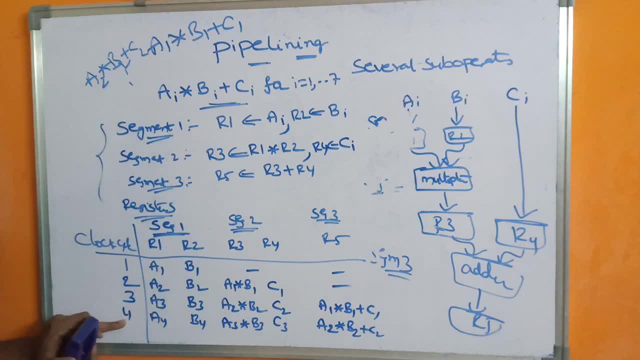 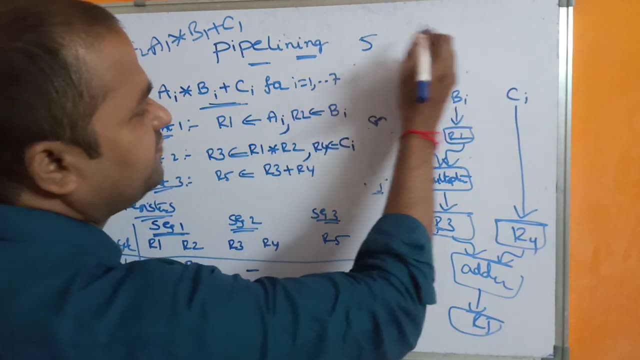 in the other set ofveltures to the output. Clook at the output. we get Cci, Ccg. so consider like that, one by one, In 5th clock cycle we will get A3 into B3 plus C3. In. 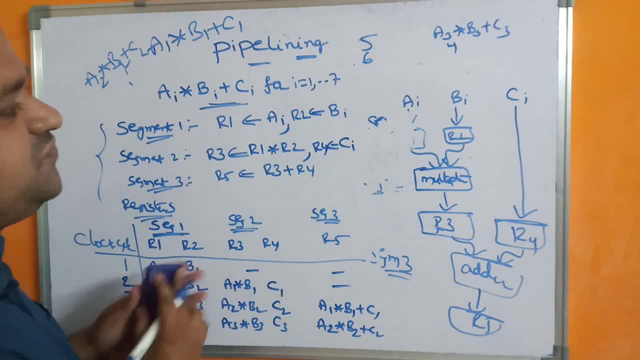 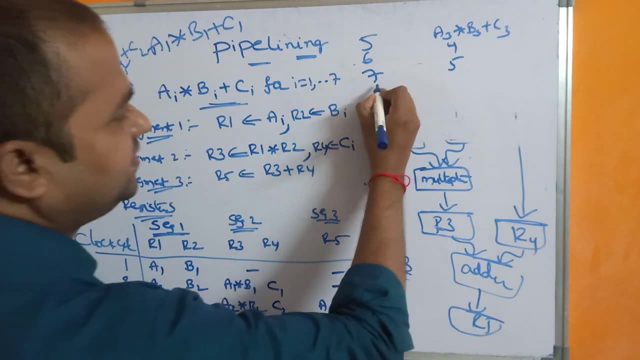 6th clock cycle we will get 4.. A4 into B4 plus C4.. In 7th clock cycle we will get A5 into B5 plus C5.. In 8th clock cycle we will get A6 into B6.. In 9th clock cycle we will 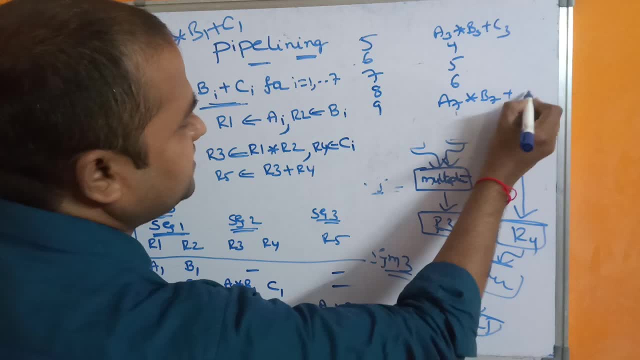 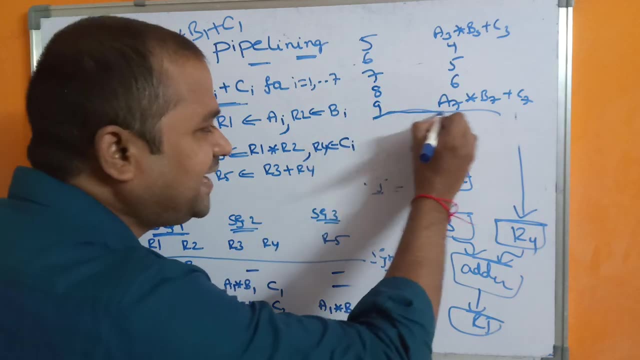 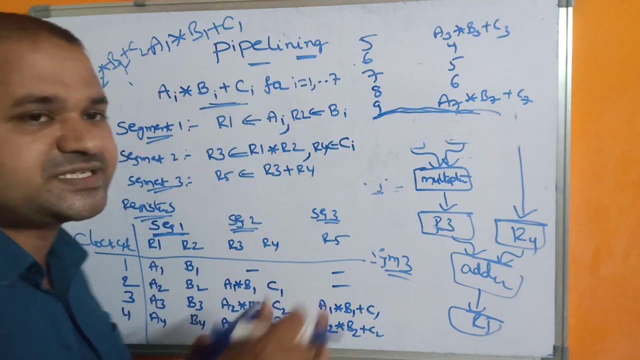 get the last one, that is, A7, into B7 plus C7. So how many clock cycles are needed in order to execute the entire process? We require 9 clock cycles. Let us assume that we executed this entire process in sequential manner, that means one by one. Then let us assume 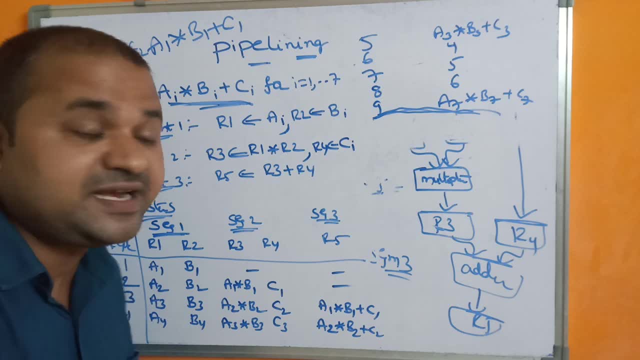 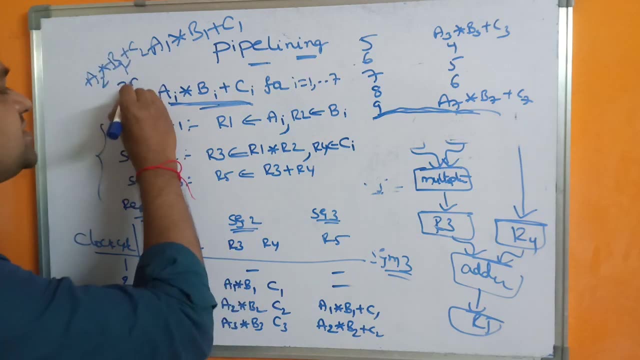 that. so for executing this process, how many segments are needed? 3 segments are needed. For executing each segment we require 1 clock cycle. So 3 segments means 3 clock cycles. So 3 clock cycles for 1 output. So 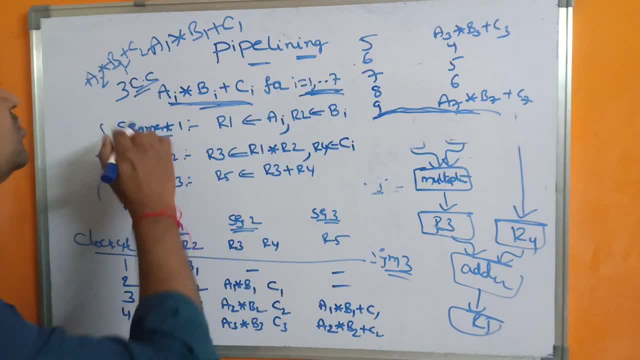 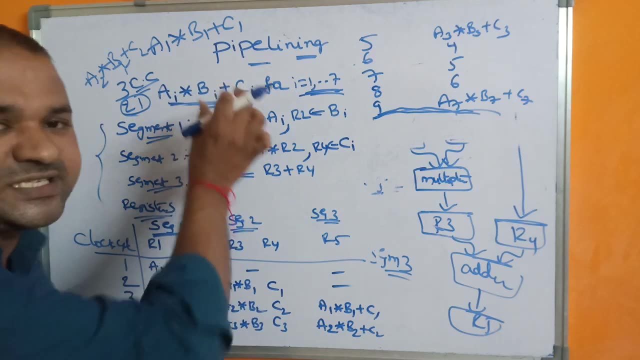 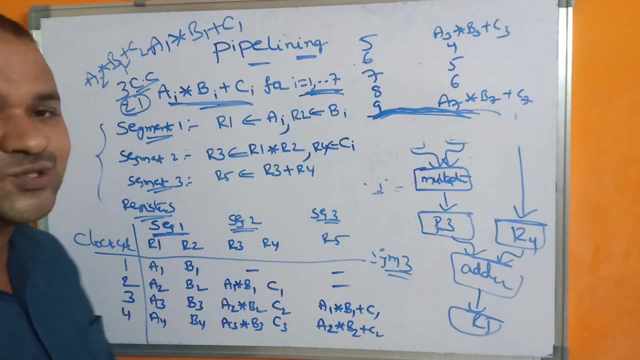 we have to get how many outputs here? 7 outputs. So 3 into 7 means 21.. So we require totally 21 clock cycles in order to execute this process in sequential manner, Whereas if we use this pipelining concept, then with the help of only 9 clock cycles only we will get the